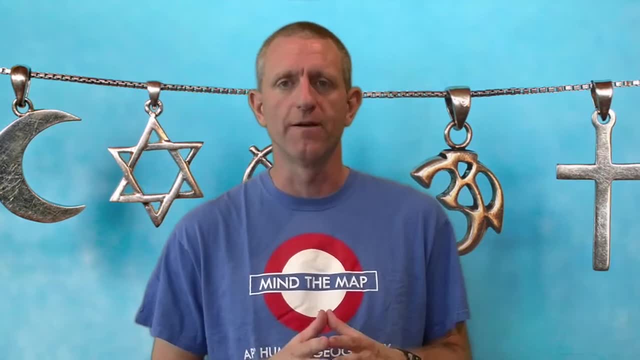 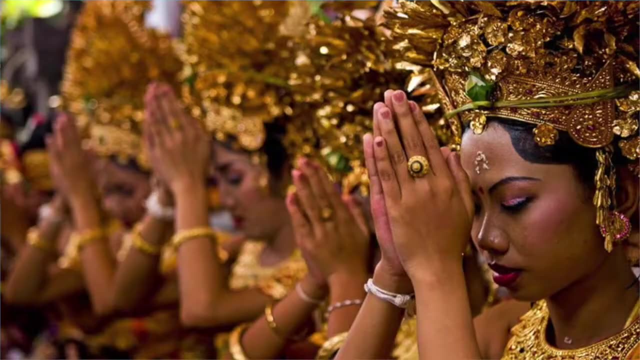 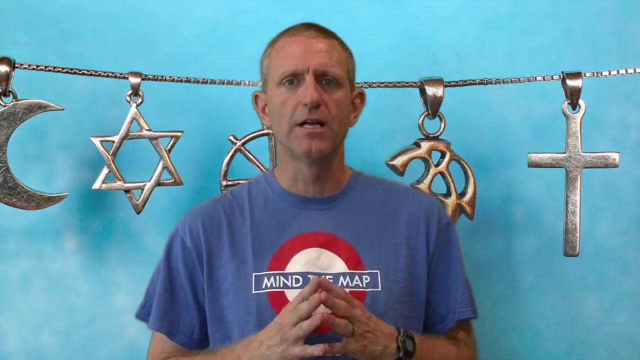 But anyway, universalizing religions, go out and seek converts. The other main category is ethnic religions, and there's two main ones that Human Geography looks at. The first is Hinduism and the second is Judaism. So let's go ahead and take a look. 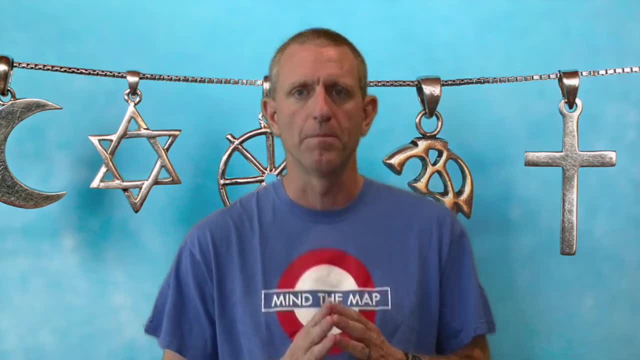 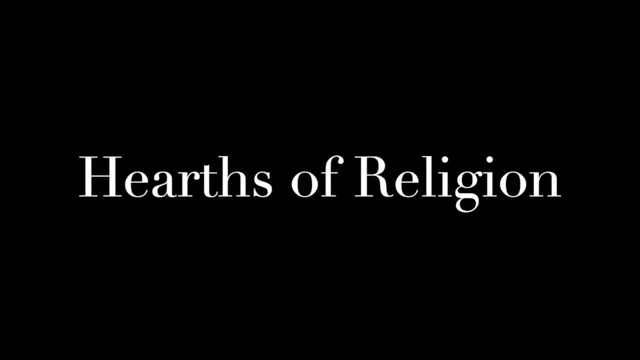 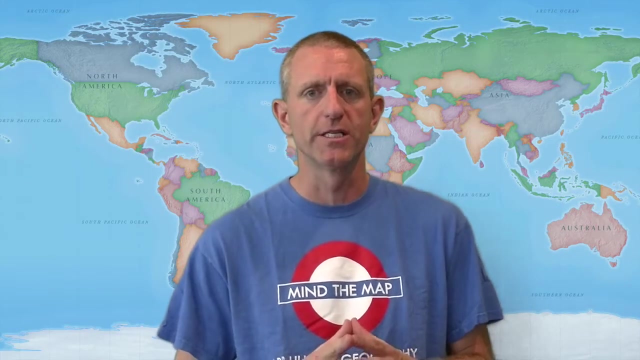 Let's go ahead and take a look at the hearths of where these religions started out from. Alright, so now let's go ahead and take a look at the hearths of these religions. So let's start with the ethnic religions. Hinduism started in South Asia, in what we call India. 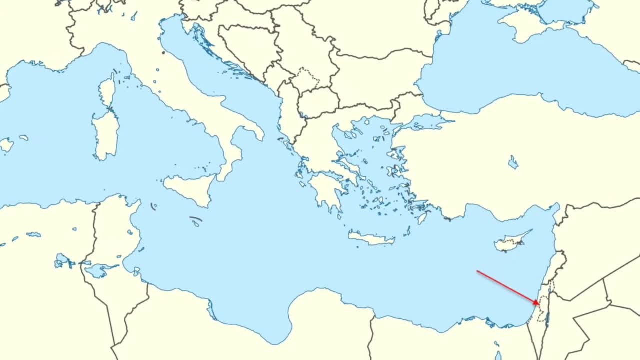 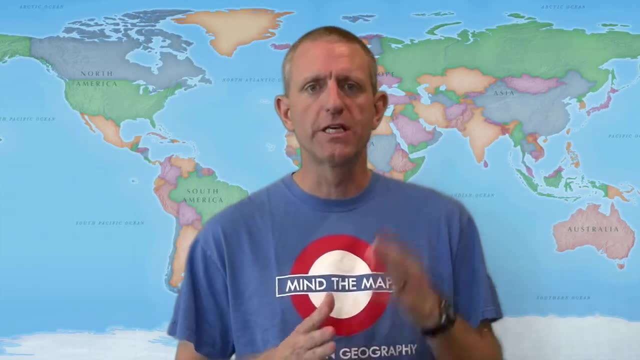 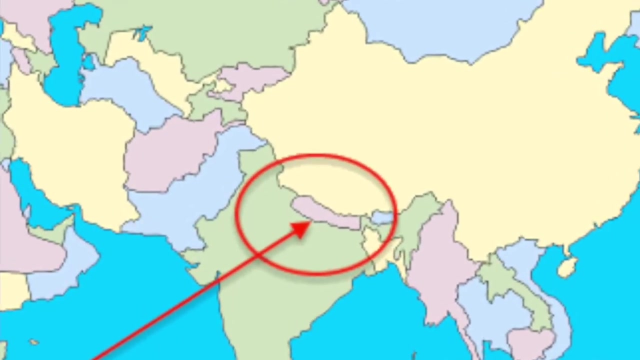 today. Judaism started in the Eastern Mediterranean area, in what is now called the Middle East, And it's now today Israel. Let's go ahead and shift our focus to the universalizing religions. Buddhism, which is an offshoot of Hinduism, started in South Asia as well. 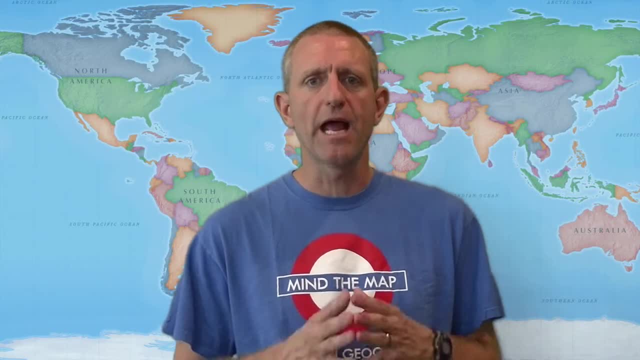 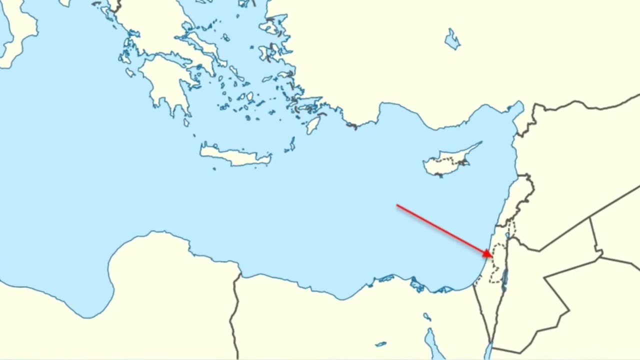 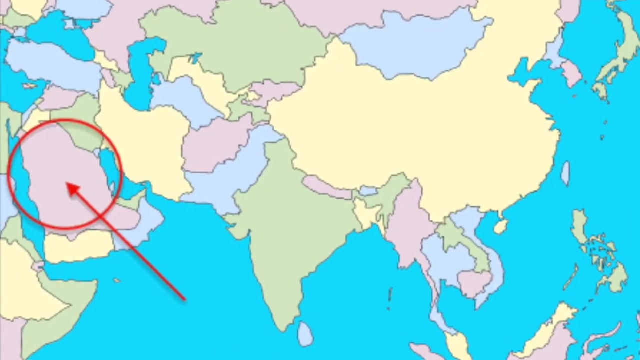 But a little bit more northeastern of where India is and what is today Nepal. Christianity, an offshoot of Judaism, started in the Eastern Mediterranean area as well, in what is called Israel. Islam started up in Southwest Asia, in what is today Saudi Arabia. And then what? 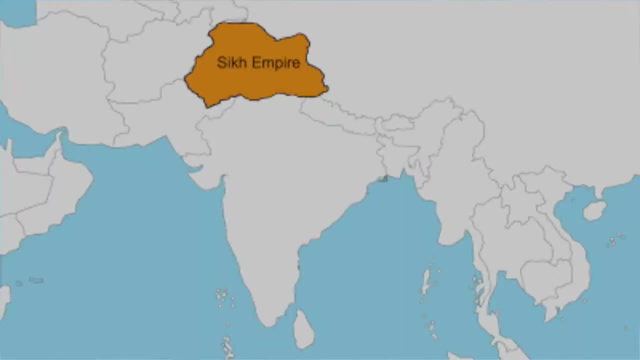 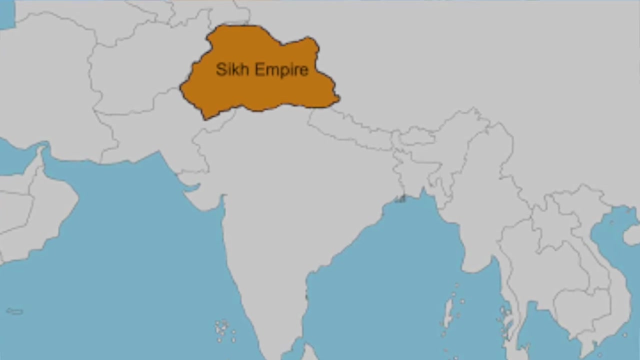 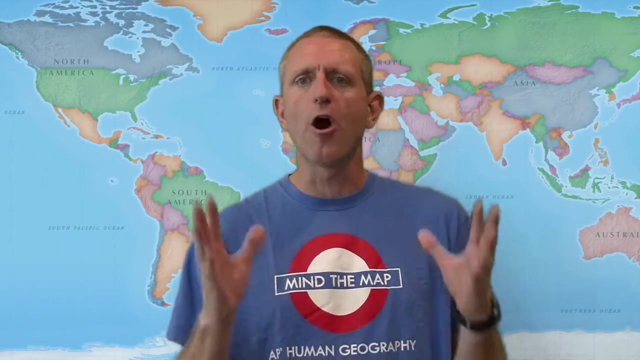 And Sikhism, which is a combination of Islam and Hinduism, started right on the border of India and Pakistan, much in the area of what is called the Kashmir region today. The one thing we would like you to notice about the religions is they all started in Asia. 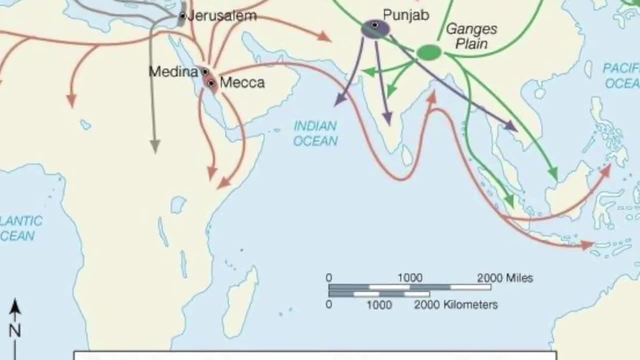 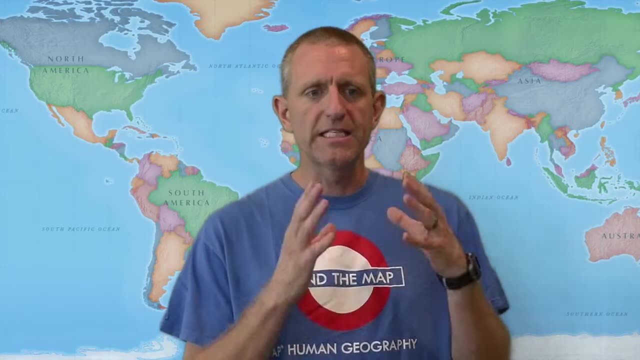 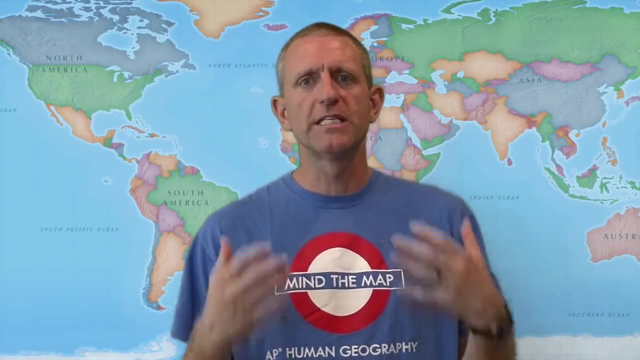 All of the major religions we cover started in South Asia or Southwest Asia, And we really want you to make the connection to that's also where there was a solid area of substantial agriculture products and also where some of the first major cities and urban areas were. 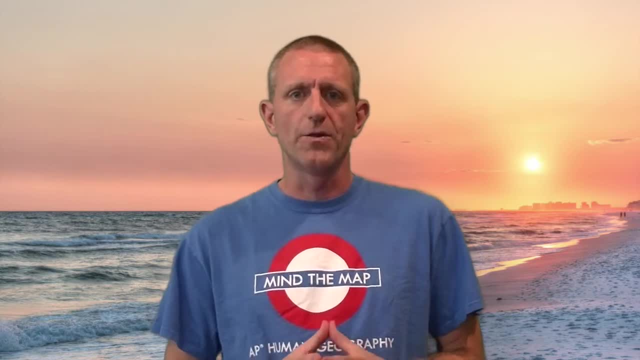 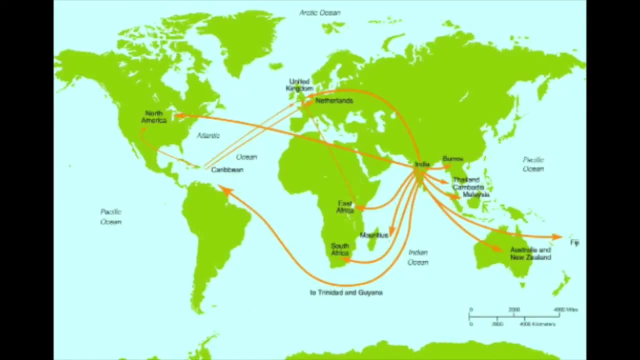 Alright, so now let's take a look at the migration of movement of all these religions. We're going to start with the ethnic religions, As we talked about previously. Hinduism is an ethnic religion, so they don't go out actively seeking converts. 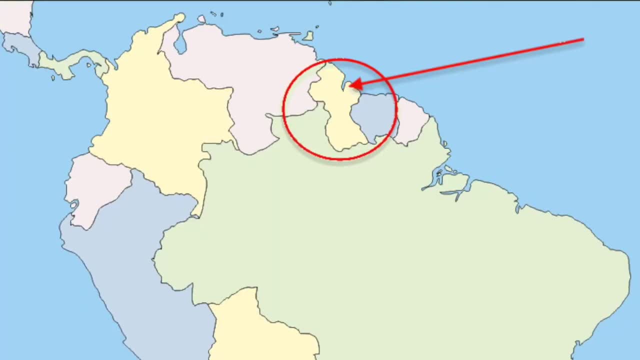 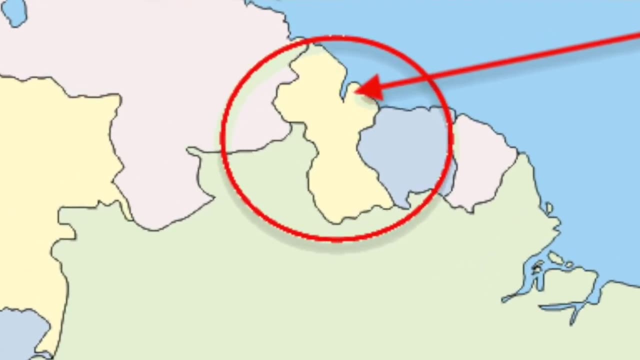 So how did Hinduism move around the world? Well, when we look at one of the beautiful maps that we give you, you can see that northern part of South America is a country called Guyana. Guyana has a high concentration of Hindus living there. 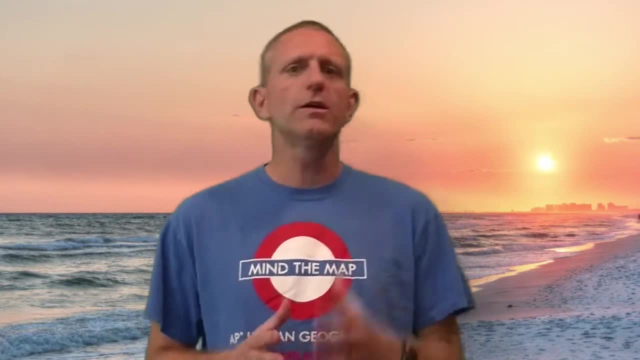 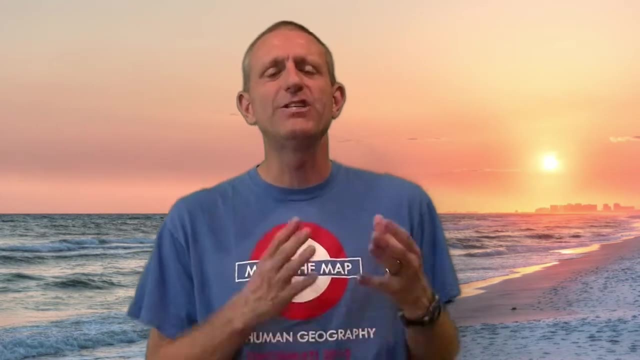 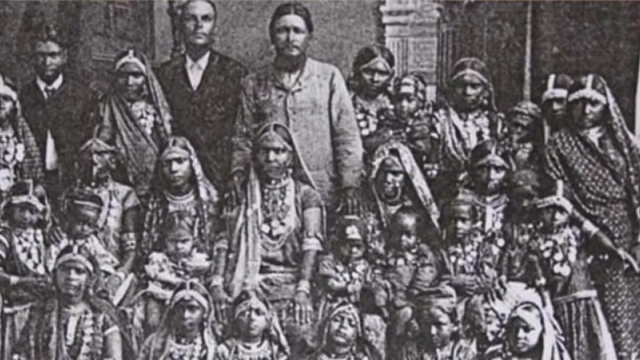 So how did that work out if it wasn't missionaries? Well, it turns out, in the 1800s the British Empire got rid of slavery. They made it illegal, But they needed cheap labor. So they went back to India and encouraged Indians to move from India to Guyana to work in the plantations and the fields. 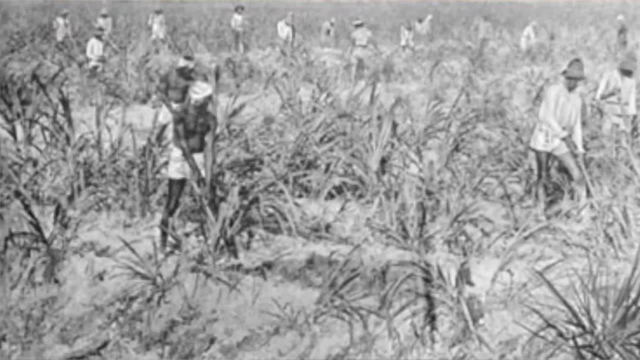 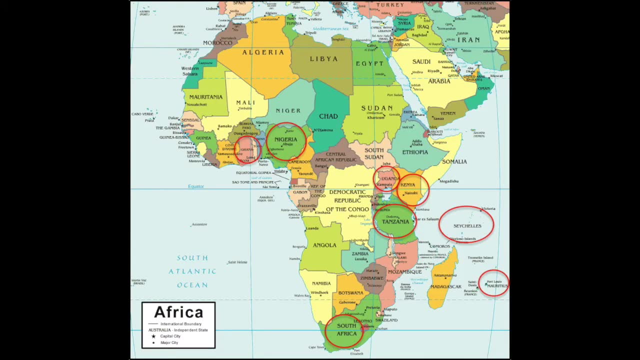 Thus relocating the people and relocating the religion. Another example of where we see Hinduism relocating is Africa. We can see pockets of Hinduism especially along the east coast of Africa, not because of missionaries moving there. We can see pockets of Hinduism especially along the east coast of Africa, not because of missionaries moving there. 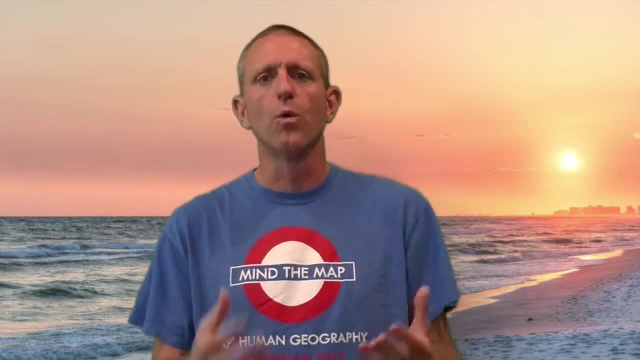 We can see pockets of Hinduism moving there, Not because ofquiera bring-in them, but because of Indians moving there to look for work, especially in the agricultural fields. Not because of India moving there to look for work, especially in the agricultural fields. 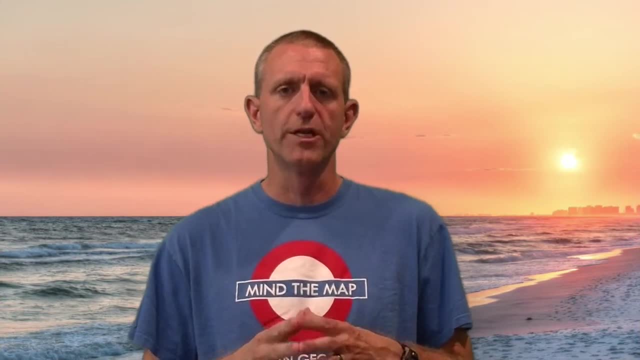 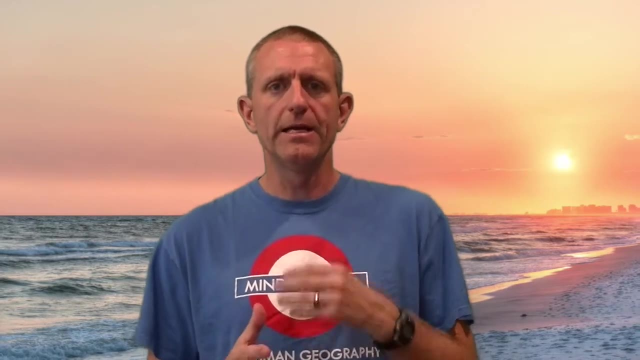 Another example of a relocation or diffusion is Judaism. Another example of a relocation or diffusion is Judaism. As we mentioned, it started in the eastern Mediterranean area. today we call it Israel. As we mentioned, it started in the eastern Mediterranean area. today we call it Israel. 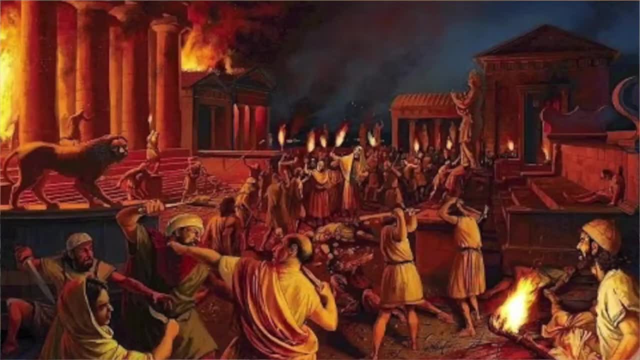 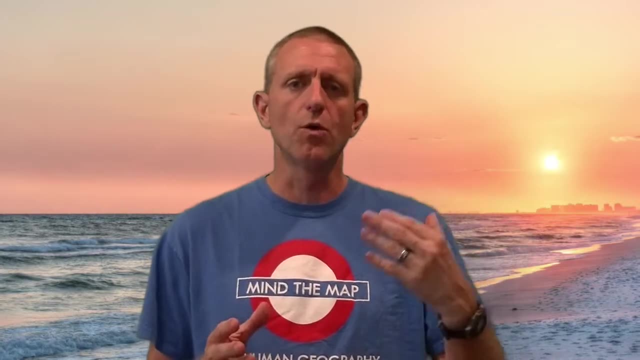 And many Jews were scattered in 아주 72 AD. This is when the Romans moved in and tore down the temple. It was called the Jewish Diaspora diaspora. Well, many of these Jews moved into Europe, Northern Africa, Russia and other areas. 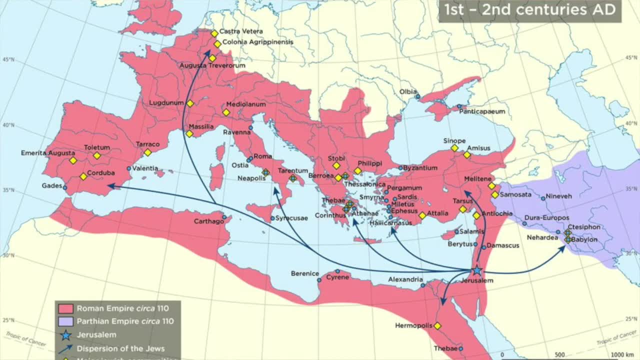 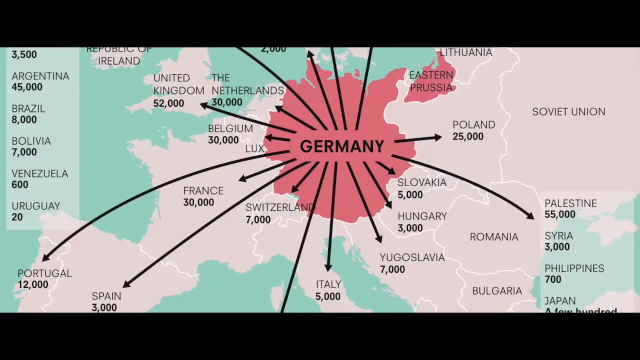 So it wasn't that the religion moved there by having missionaries go out. It moved there by people relocating and bringing their religion with them. We see this again happen in the 1930s, as Jews were fleeing the Nazis. We see it move into places like the United States and Canada. 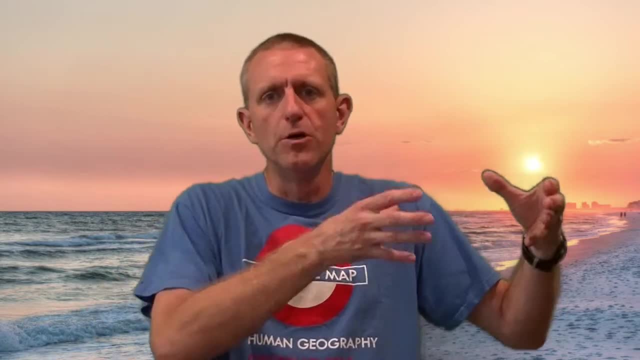 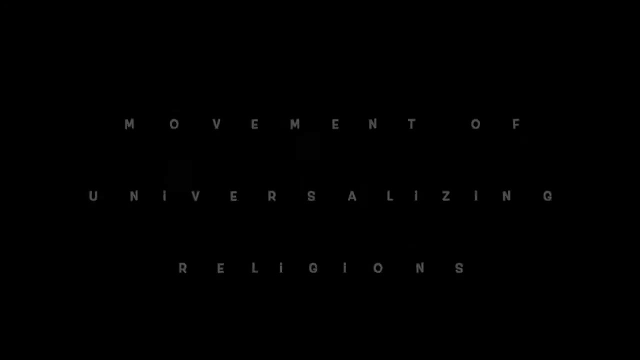 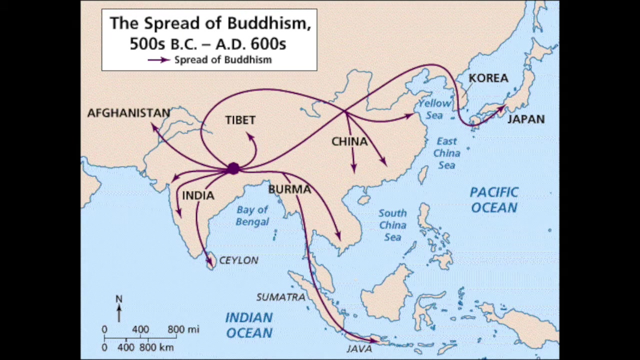 and other countries. So the people picked up, moved and relocated the religion with them. All right, so let's go ahead and start looking at our universalizing religions. Buddhism and Sikhism spread through relocation, diffusion and expansion. diffusion Because they 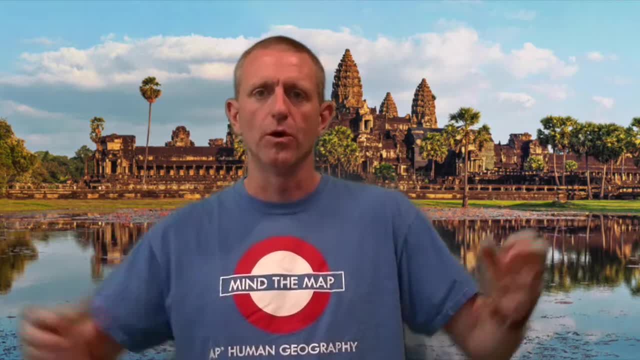 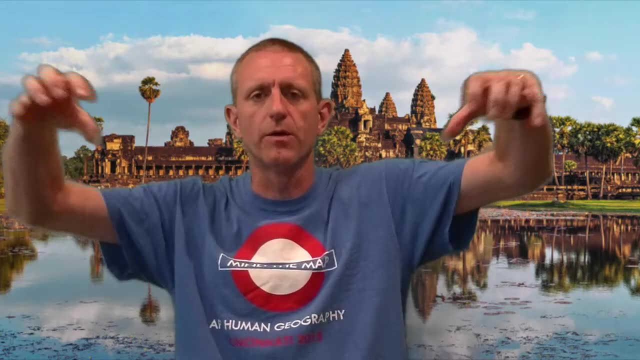 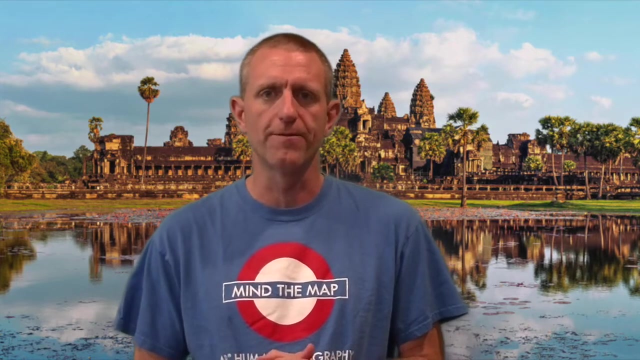 will go out and recruit people in. it expands outward. But also as people that are Buddhist and Sikh go out and move and go to new regions, they relocate the religion as well. Christianity is very well known For expansion, diffusion and relocation. diffusion: Explorers since the 1400s have 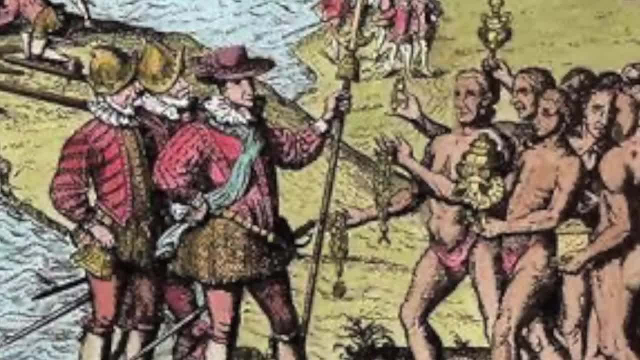 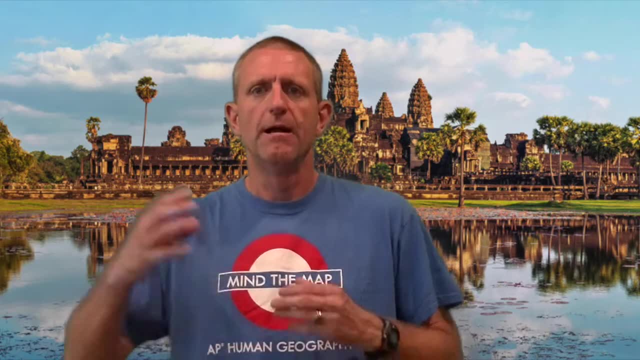 gone around the world conquering areas and forcing people to join or to convince people to join. So we see that as the expansion, or contagious diffusion, by going out and actively recruiting people in, either by force or by being nice and saying, hey, do you want to? 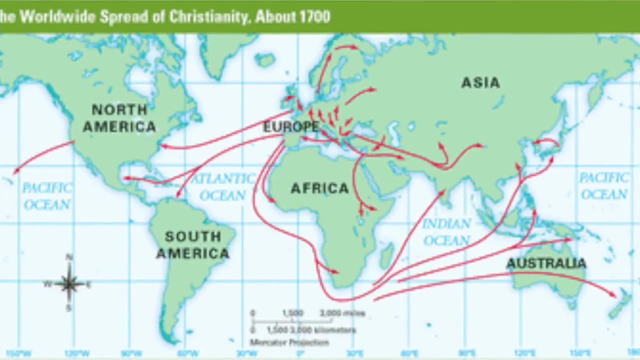 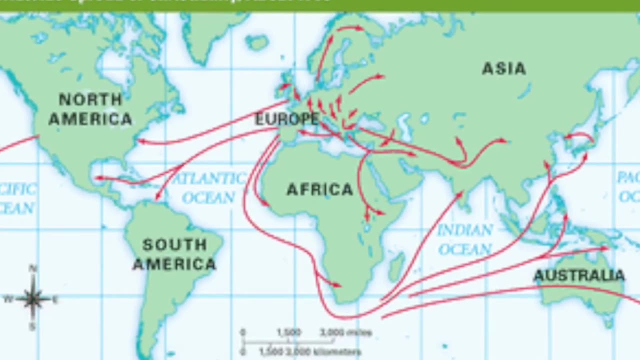 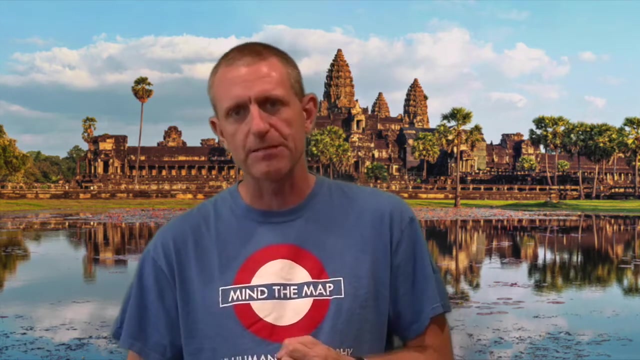 join us. We also see it through relocation diffusion. As the Spanish moved into the Americas, the Portuguese, the British, the French, they brought the religion with them and then spread it out from there. So we have seen Christianity use relocation diffusion and expansion diffusion. 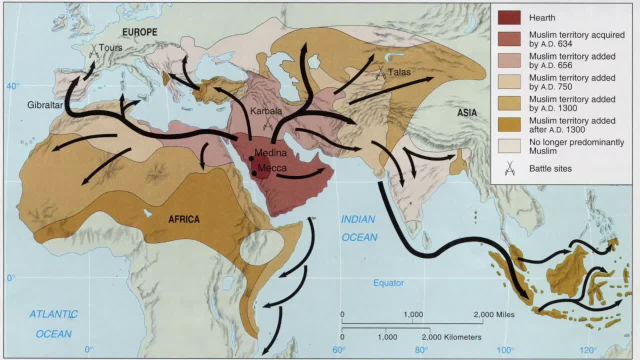 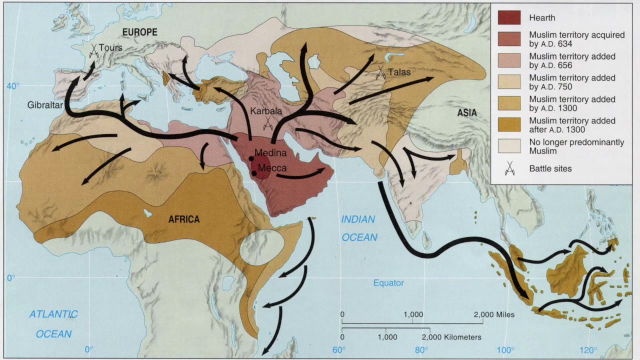 The same with Islam. Islam originally spread out from Saudi Arabia into northern Africa, east, towards India and up into parts of the Balkan Peninsula through contagious diffusion, But then also at that same time, we see a lot of Muslim traders going to places like Indonesia, Africa. 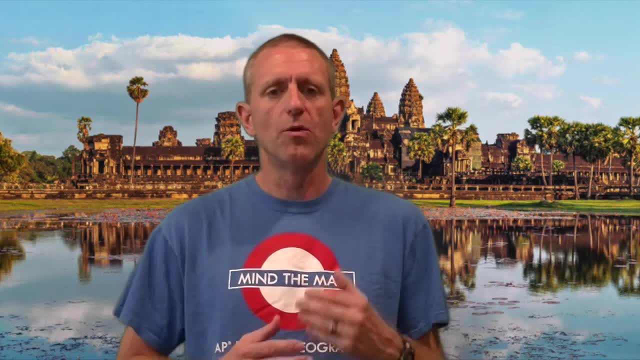 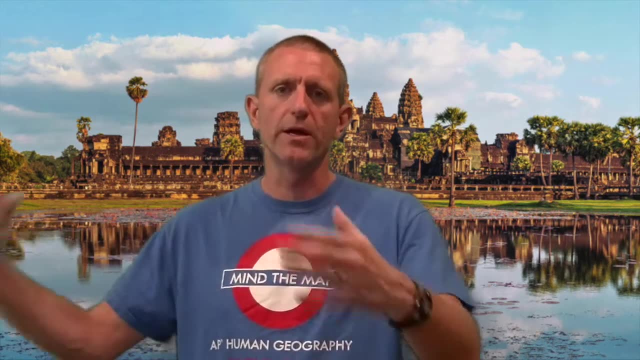 and other parts of the world, taking the religion with them. So that's where we see the relocation diffusion. As these traders went out and made settlements, they then too tried to spread the religion from there, just as Christianity did. So when we look at universalizing religions, 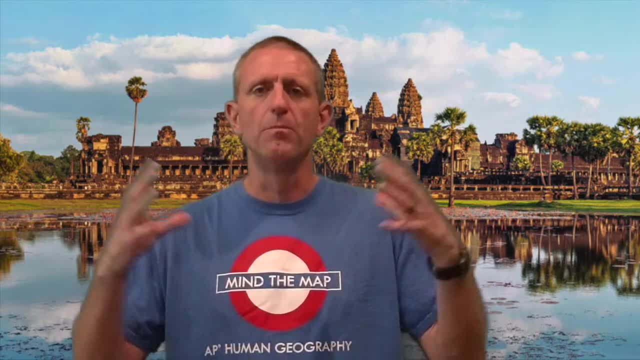 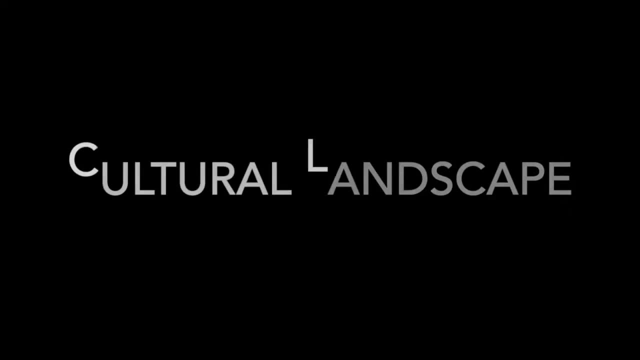 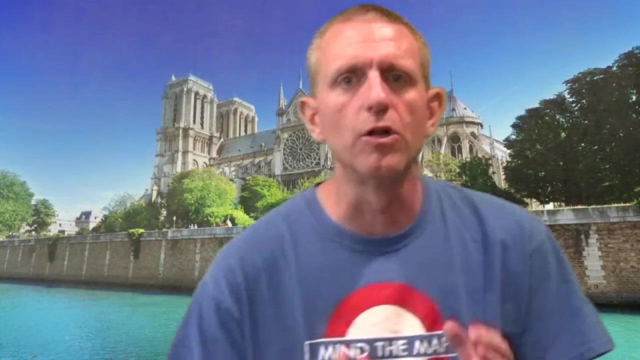 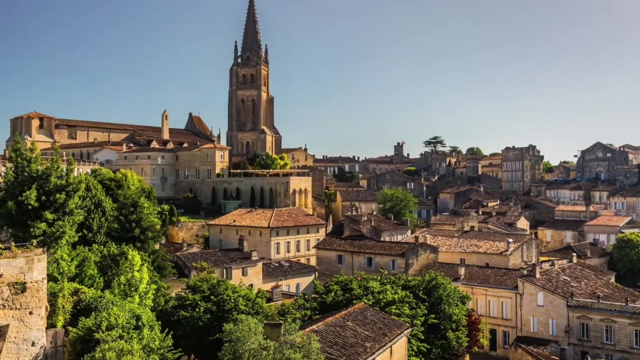 they can use both relocation diffusion- by people moving and creating settlements- and contagious diffusion, by trying to convert people around them. Our last topic we're going to look at is landscape, and religion has had a huge impact on the landscape. When we look at Christianity, Christian churches have always been a very big focal point of 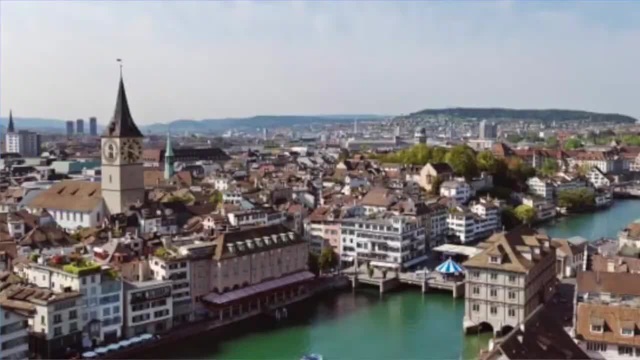 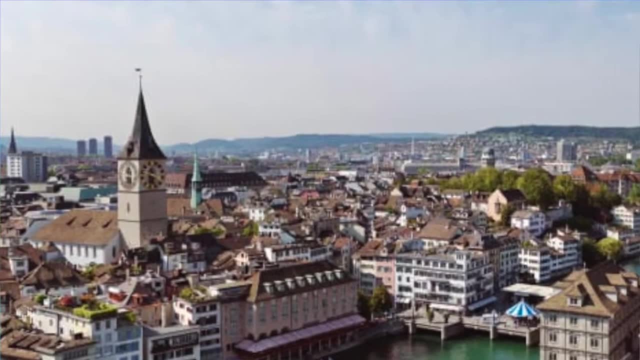 their communities throughout Europe and other parts of the world. as they spread out, Churches with huge steeples on them are the ones that have the greatest impact on their communities. The steeples on top usually were the tallest building in communities for the longest time. 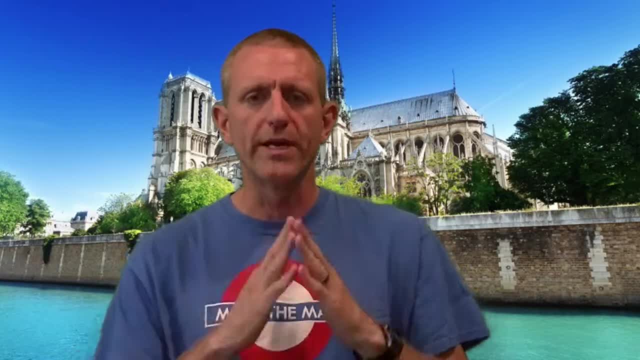 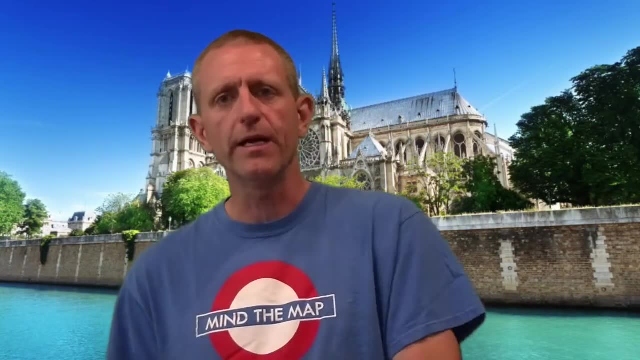 They also had buildings that were typically a little bit of a pointed roof area. That was to make the snow run off so that it would not weigh down. However, when we go to the Mediterranean regions in Eastern Europe, we can see where the Orthodox Christians adopted. 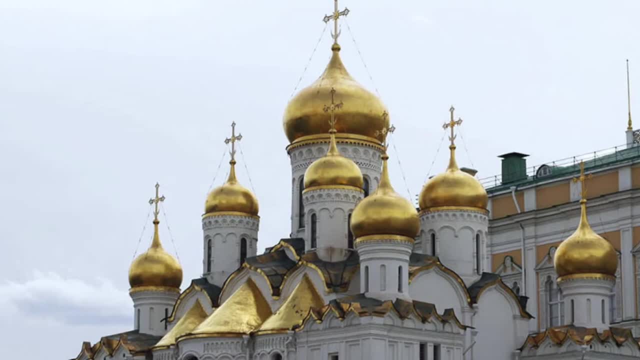 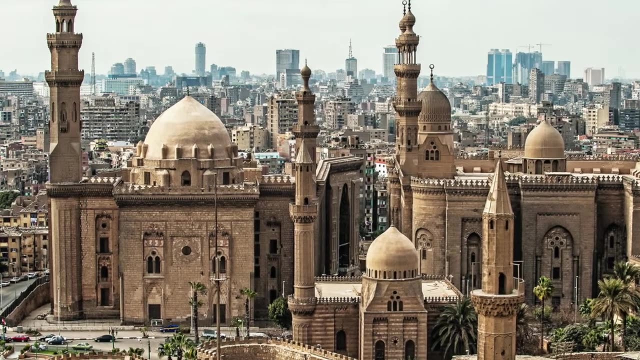 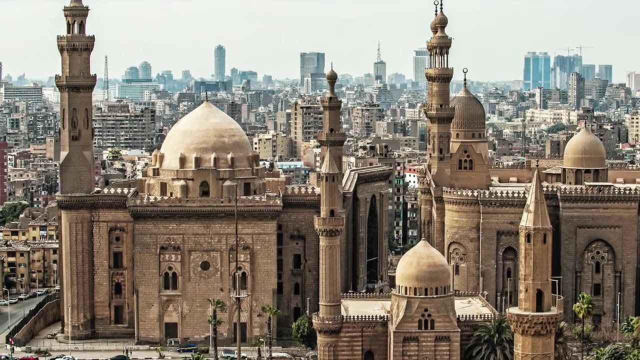 more of a Middle Eastern. look to their churches when they spread out. Like Christianity, Islam also had buildings that were usually in the middle of town and very large, and were a big focal point of the vision. These large mosques had minarets around them that were used to. 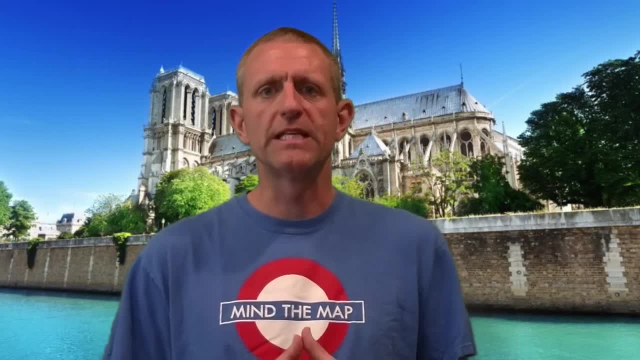 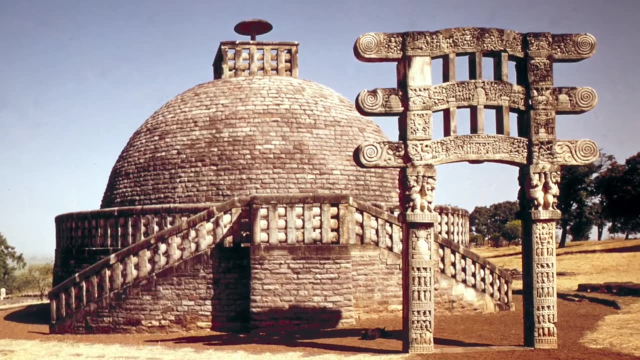